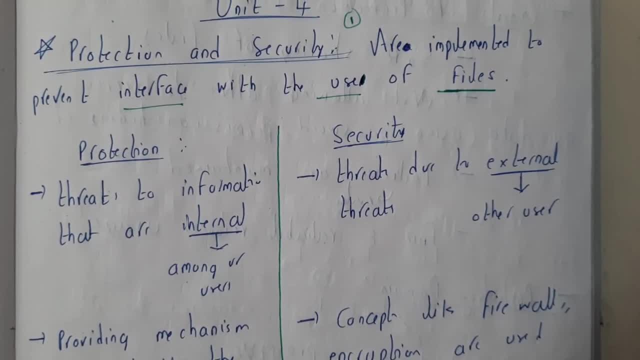 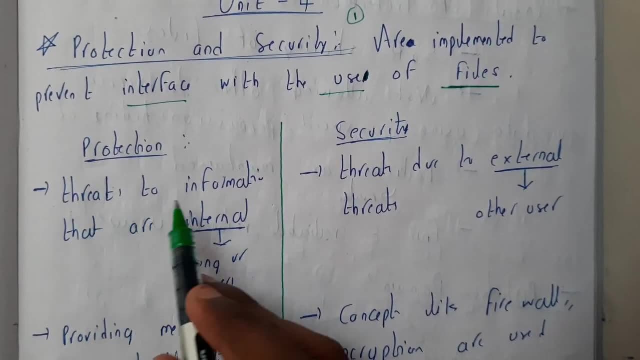 protection and security. After that, we will be starting with goals of protection and we will be continuing to protection and then we will be starting security. Okay, So protection: threats to information that are internal, Threats due to information that are internal. 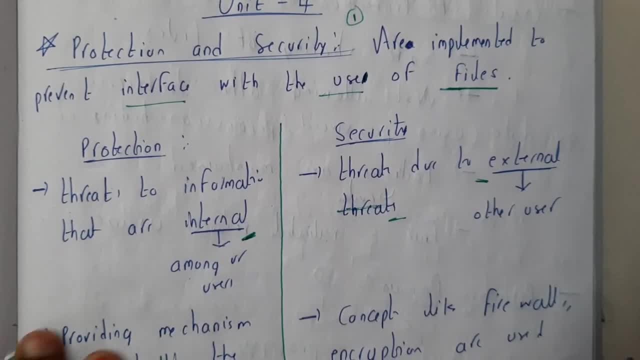 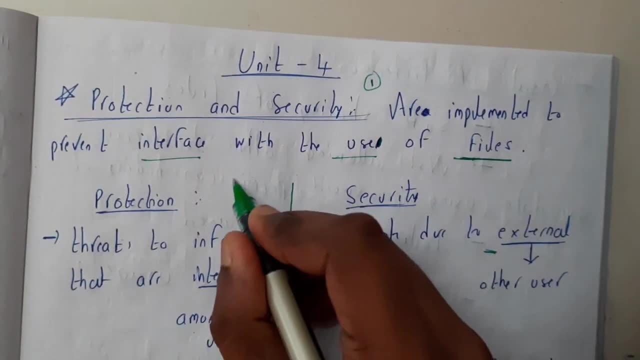 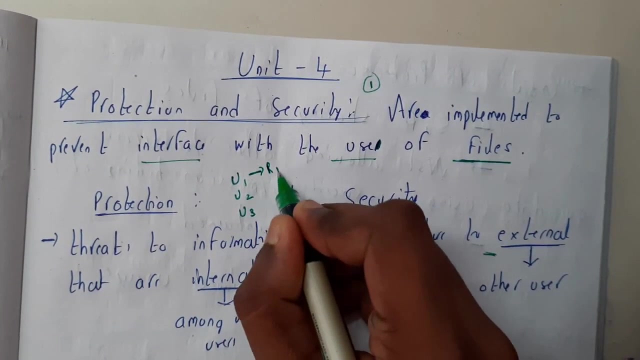 external, external or external threats. okay, so your doubt is now: what is internal, what is external? so protection, if let us assume there are n number of users- one, sorry, let us assume three users, so there are three users, the user one should only access resource one where user two and three can access. 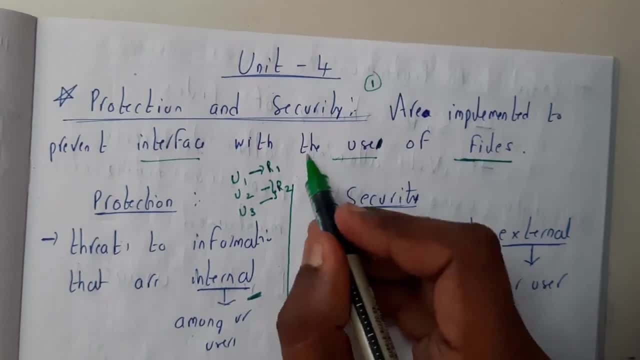 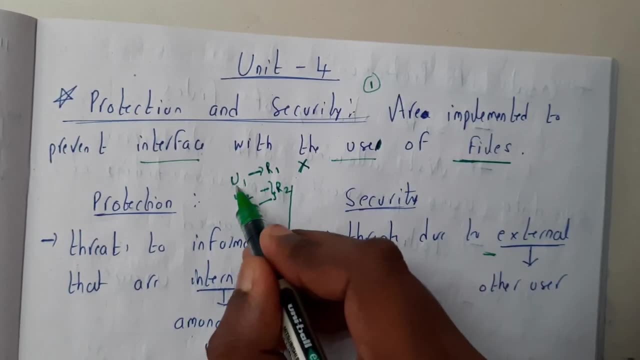 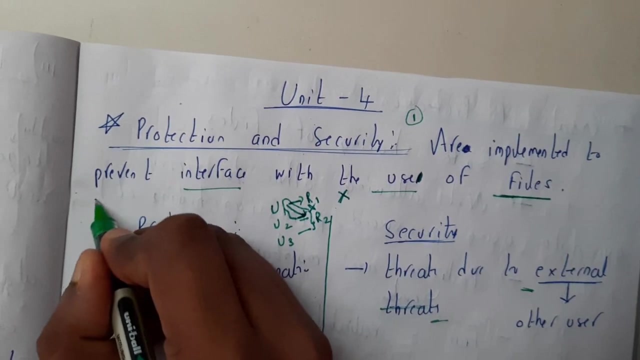 resource two: fine, and there is one more, user X, who is completely out of our our system. so, basically, if user one is accessing our one, if user one tries to access our two, as he is not having any permissions, if he tries, then this should not allow because, okay, let us assume that your father files are there. parent. 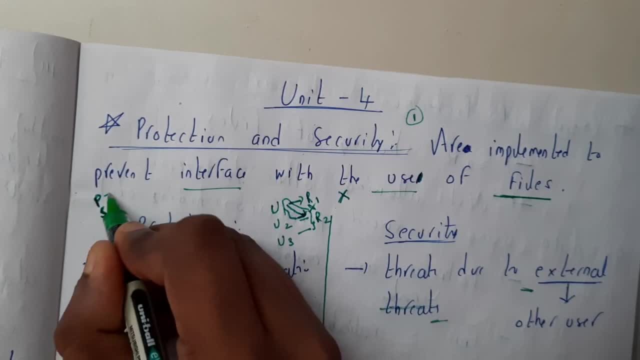 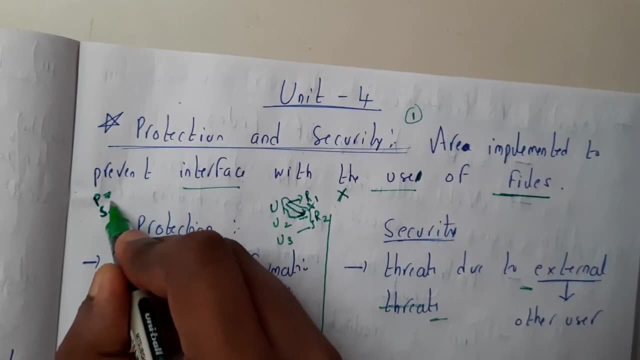 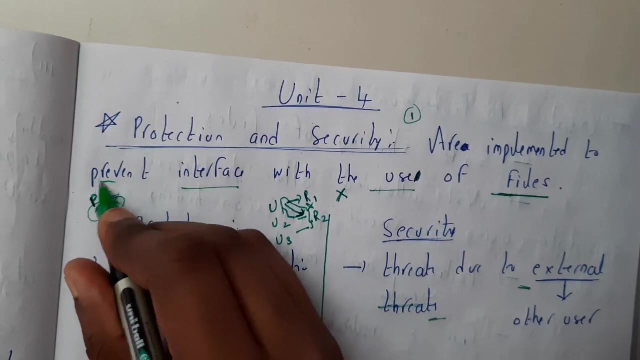 and you are the son. so your father is having many files which are really important according to his job or according to the bank balance, bank details and everything. will they allow your son or you to access them? mostly no. so that this, to make this happen, we need 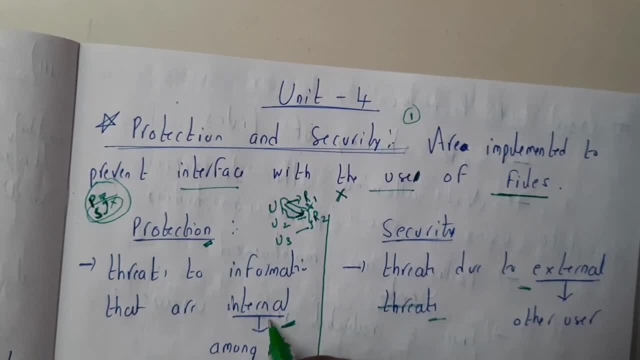 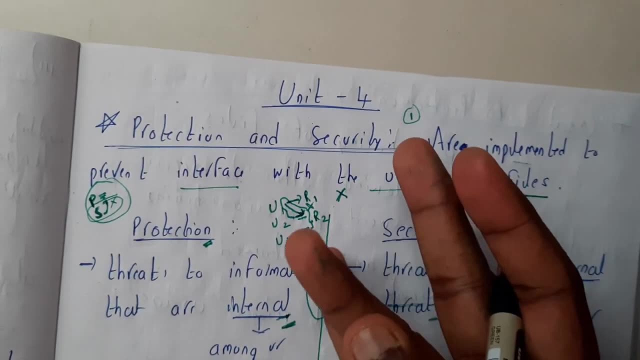 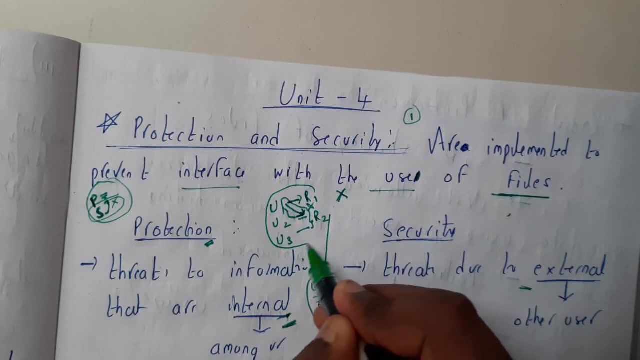 the concept of protection guys. so internal threats are nothing but among your users only. you need to have some protections. those are nothing but access permissions, access rights that we will be discussing, don't worry so security. security is external, so you are using your files, so this is your system. 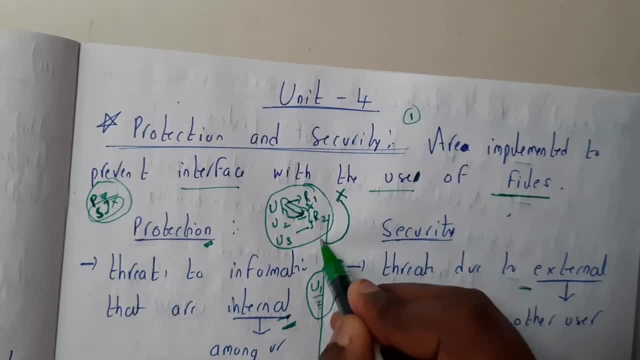 unfortunately, a guy from some are some other system tries to enter your system. you are using your files, so this is your system. unfortunately, a guy from some other system tries to enter your system and read your files. to avoid this, we will be using the concept of security. 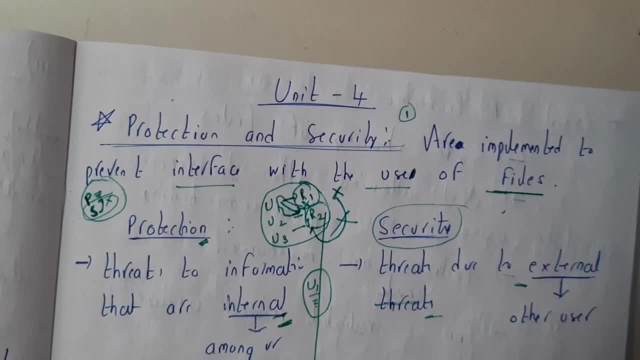 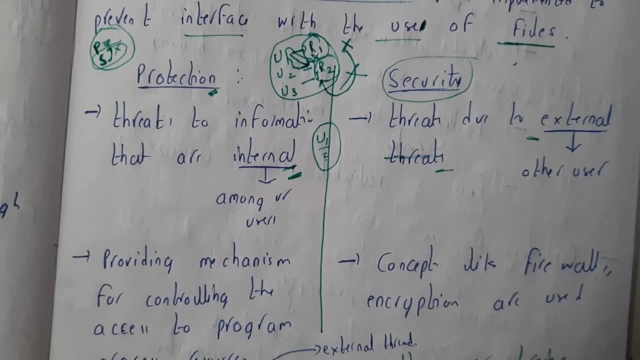 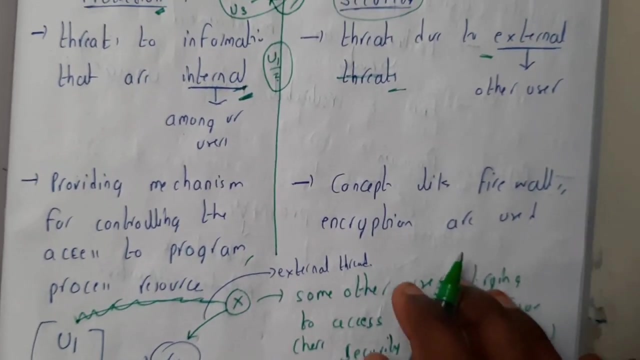 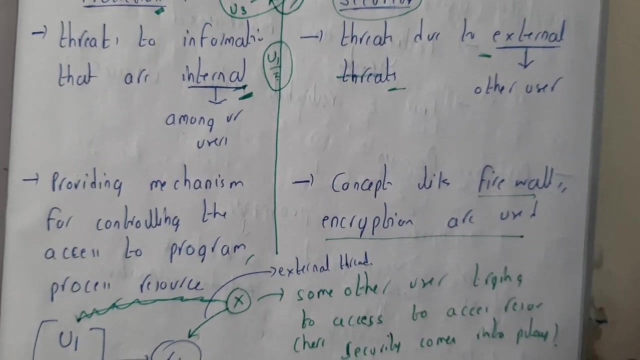 fine, so I hope everyone got a clean idea on differences between protection and security. okay, so protection provides mechanism for controlling the access of program or process or resources. fine, so security concepts like firewall and encryptions are used here. okay, so I hope everyone got a small idea. 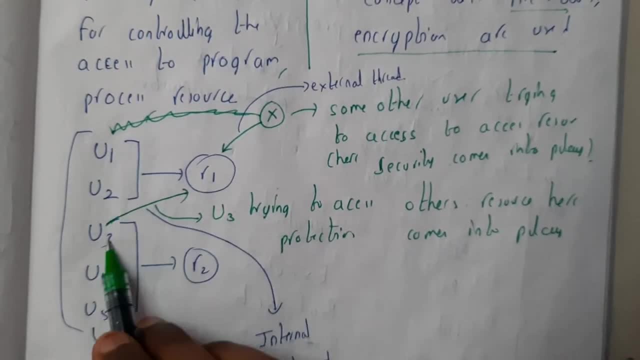 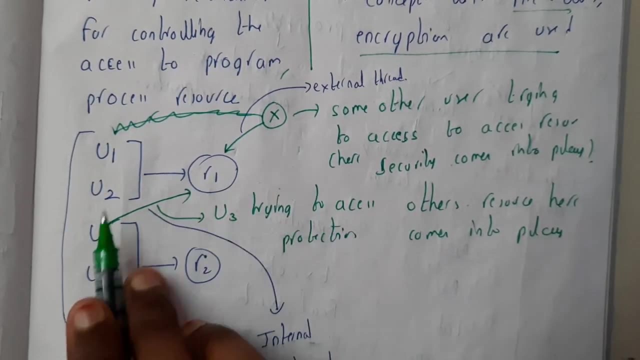 so that's what I've just written here in the form of a small example. so let us assume you 1, you to you 3, you 4, you 5, other five users in a system, and r 1, 1 are two other resources, and here X is an unknown guy.